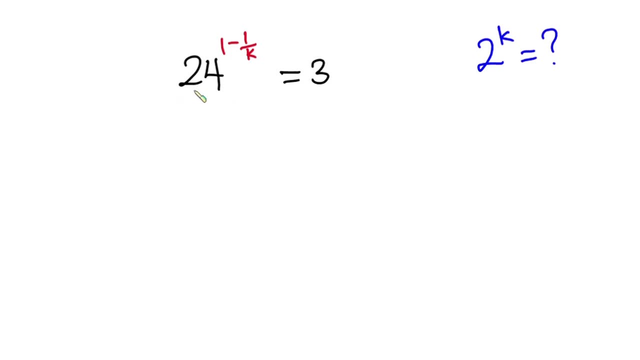 Hello everyone, In this video we have this nice problem: We have 24 to the power 1 minus 1 on k and this is equal to 3, and we have to find the value of 2 to the power k. We will solve this. 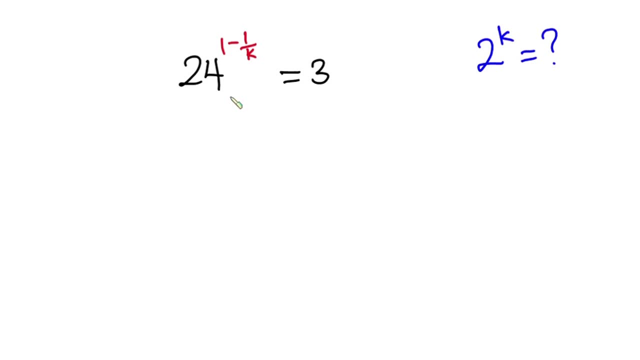 problem in a step-by-step manner, without missing any step. but before we begin, if you are new here, please do me a favor by subscribing to this channel. It is free, there's no charges on that and you can change your mind at any time. Thanks a lot for subscribing. Now let's get started. 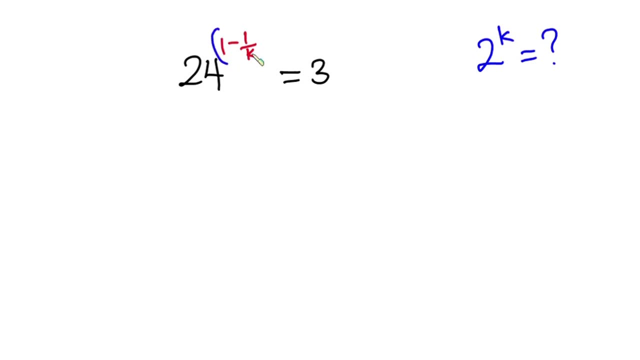 First of all, I'll combine this exponent over here, and to do that, they need to have the same denominator. Okay, so I'll rewrite this exponent as k on k, which is the one over here, then minus 1 on k, and this is equal to 3.. All right, so now, since they have the same 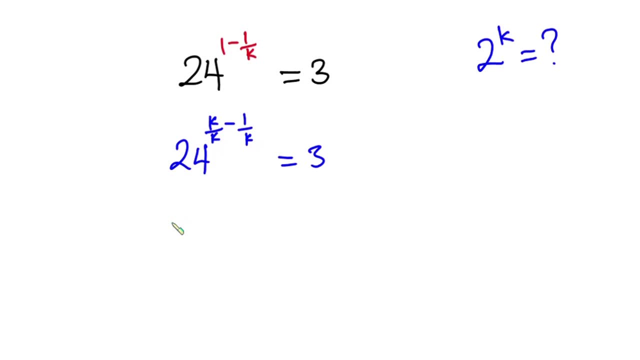 denominator. we can easily combine them. So we have 24 to the power k minus 1 over k, and this is equal to 3.. All right, so the next step is that we are going to take the k power on the both sides of the equation, All right. so here we have 24 to the power k minus 1 over k times k, and this is equal to. 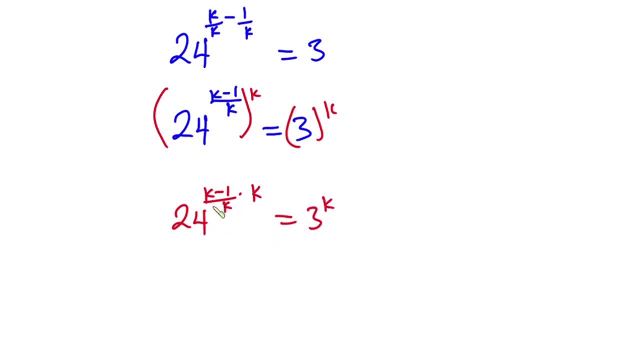 3k. All right, so straight away you can see that this k will cancel this. Now we have 24 to the power k minus 1 is equal to 3 to the power k. Okay, and note that this 24 to the power k minus 1. 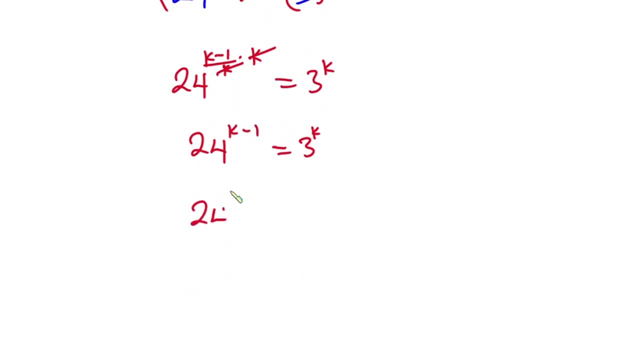 is also the same as 24 to the power k over 24, and this is equal to 3 to the power k. All right, so now let's cross multiply, So we have 24 to the power k is equal to 24 times 3 to the power k. 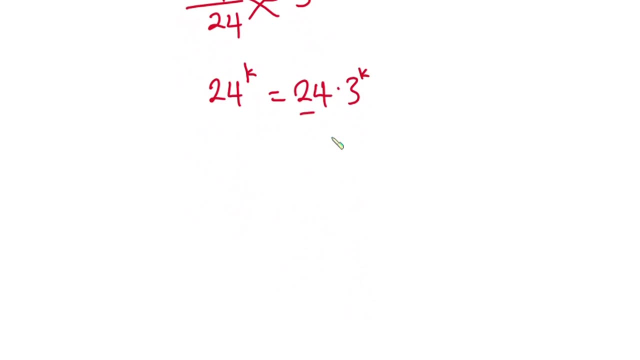 Okay, so from here we can divide each side by 3 to the power k, so that this one will take care of this. Now, if you have a to the power m over b to the power m, this is the same as a over b, all to the power m. Okay, so I'll rewrite this in this form. so we have. 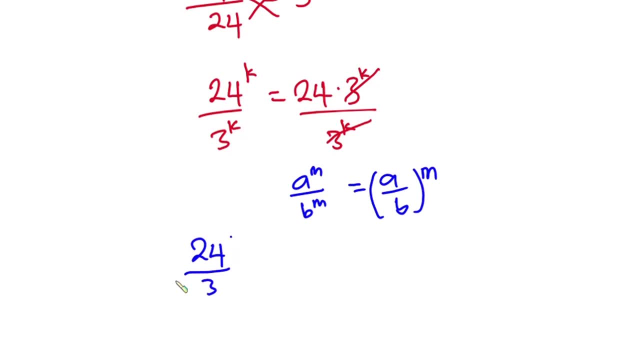 24 on three, or to the power, k, and this is equal to 24.. All right, so from here, 24 divided by 3 is nothing but 8.. Then this k, and this is equal to 24.. Since we are looking for 2 to the power, 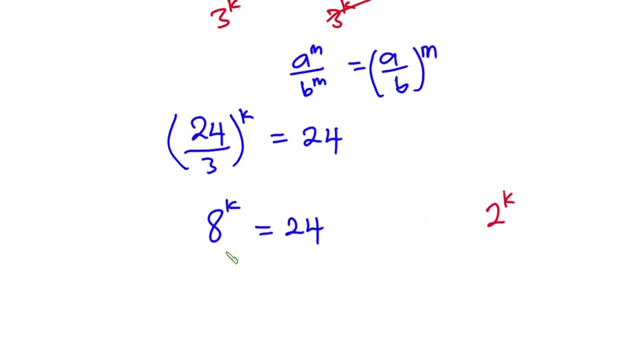 k. I will write this 8 in this form: All right, so from here we have 2 to the power, 3 to the power. k is equal to 24.. All right, so if you have a to the power m, and this is also the same as a to the power, 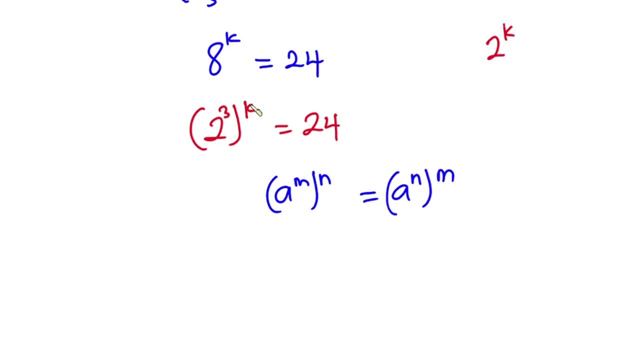 m. Okay, so I will interchange 3 and k. so we have 2 to the power k, 3 over here, and this is equal to 24.. since we are looking for 2 to the power k, i will take cube root on both sides. all right, so that this one will cancel this. now we have 2 to the power k. 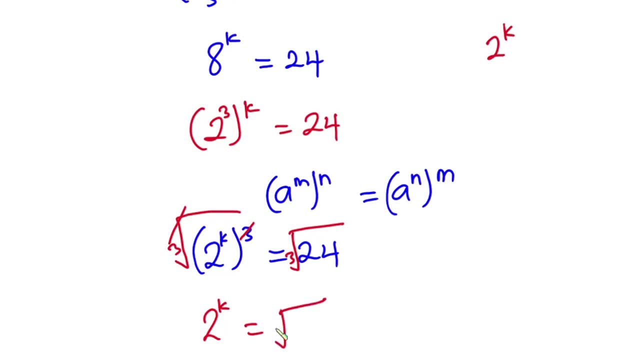 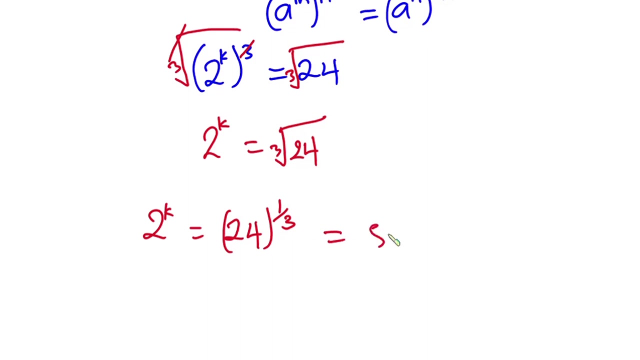 is equal to the cube root of 24. all right now we know. 2 to the power k, but we can simplify this further. this is also the same as 24 to the power one third. okay, this is the same as cube root. and this is also the same as eight times three, or to the power one third. all right, now i can rewrite. 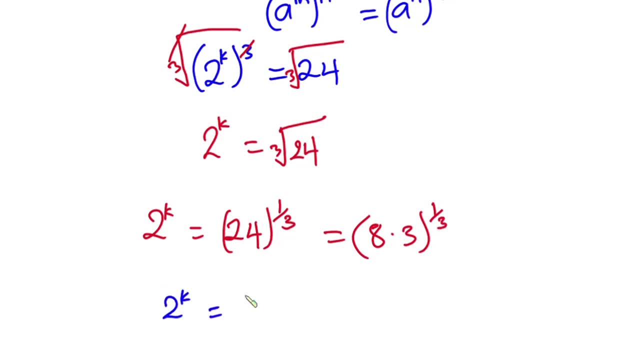 this as two to the power three times three or to the power one third. okay, now this is also the same as two to the power. k is equal to two exponent three times one on three times three to the power one on three, so that this theory will cancel this. now we have two to the.